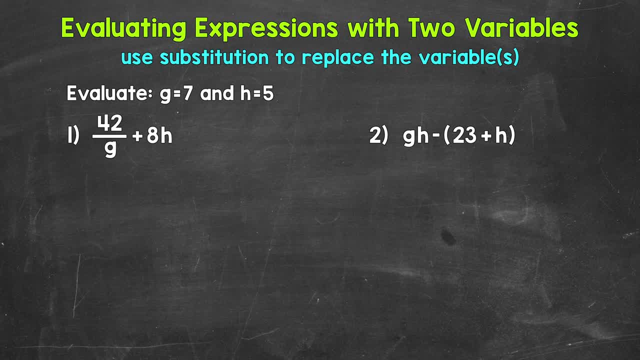 we need to do is replace or plug in the given values for the variables. This is called substitution. So let's plug in 7 for g and 5 for h and rewrite this expression. So we have 42 over g. Let's plug in 7 for g plus 8h, So 8 times h. Let's plug in 5 for h. Now we can evaluate. 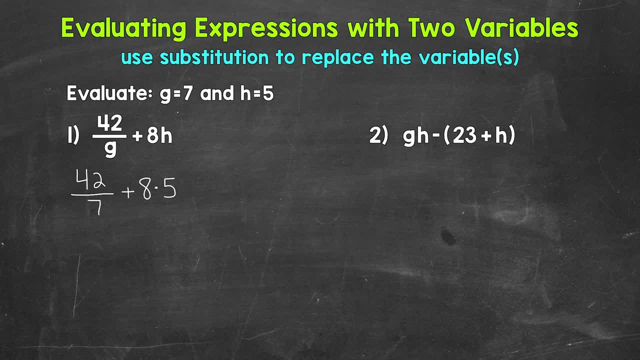 So let's figure out what this equals. Since we have more than one operation, we need to use the order of operations, So let's plug in 7 for g and 5 for h. Now we can evaluate, So let's plug in. 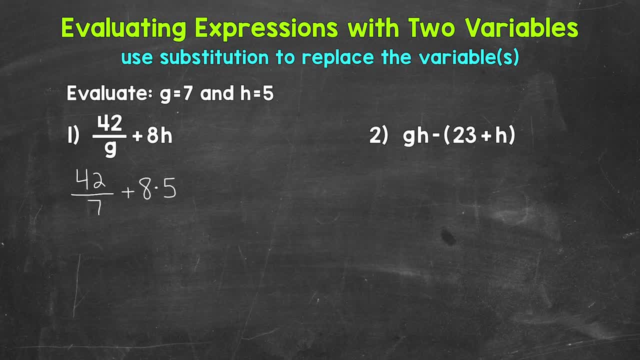 7 for g and 5 for h. Now we can evaluate. So let's plug in: 7 for g and 5 for h. Now we need to use the order of operations PEMDAS to work through this. So parentheses, exponents, multiplication and. 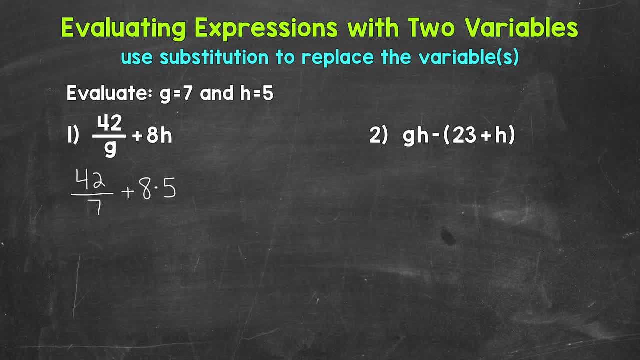 division, then addition and subtraction. As far as the order of operations, we don't have any parentheses, We don't have any exponents, So the next priority would be multiplication and division. We have both. So what we can do, we can work from left to right, So division comes. 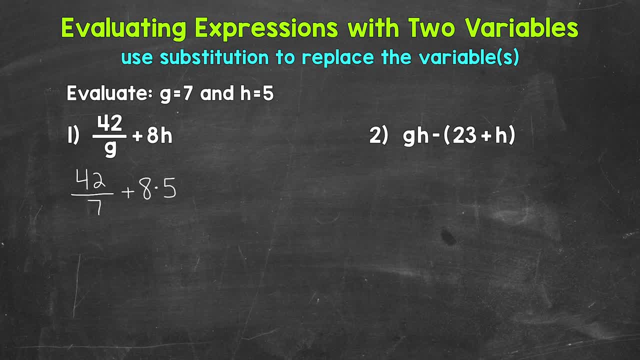 first. So let's do 42 divided by g plus 8h. So let's plug in 7 for g plus 8h. Now we can divide it by 7 to start off. 42 divided by 7 equals 6.. Bring down everything we did not use. 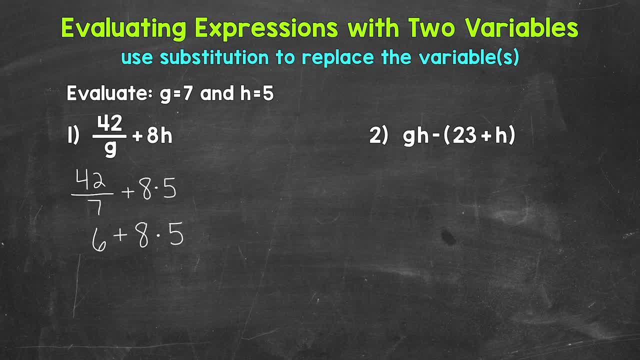 So the addition sign, the 8,, the multiplication sign and the 5.. Now we have addition and multiplication. Multiplication comes before addition, So let's multiply next 8 times 5, that equals 40.. Bring down the addition sign and the 6 that we did not use. 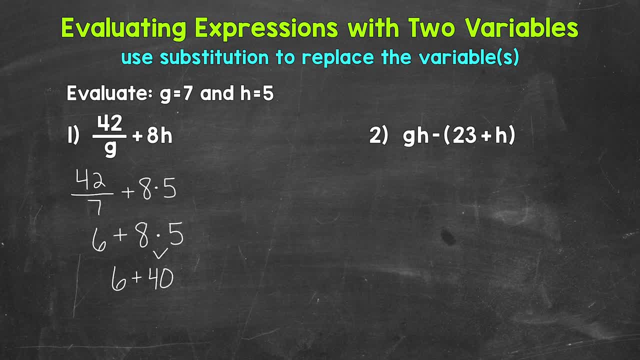 And we end with addition. So we have 6 plus 40. That equals 46. So the value of this expression is 46 when g equals 7 and h equals 5.. Let's move on to number 2, where we have gh, So g times h. 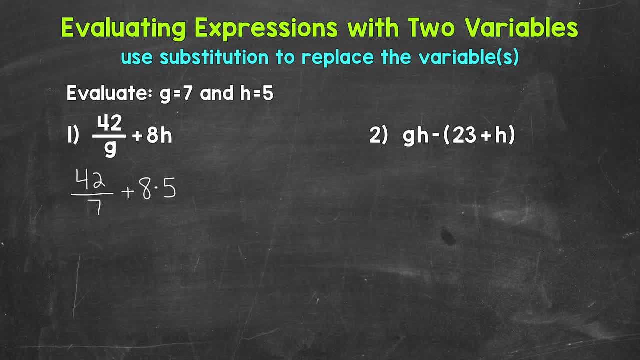 division, then addition and subtraction. As far as the order of operations, we don't have any parentheses, We don't have any exponents, So the next priority would be multiplication and division. We have both. So what we can do, we can work from left to right, So division comes. 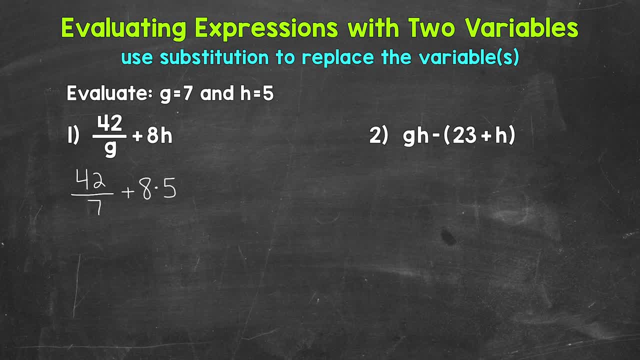 first. So let's do 42 divided by g plus 8h. So let's plug in 7 for g plus 8h. Now we can divide it by 7 to start off. 42 divided by 7 equals 6.. Bring down everything we did not use. 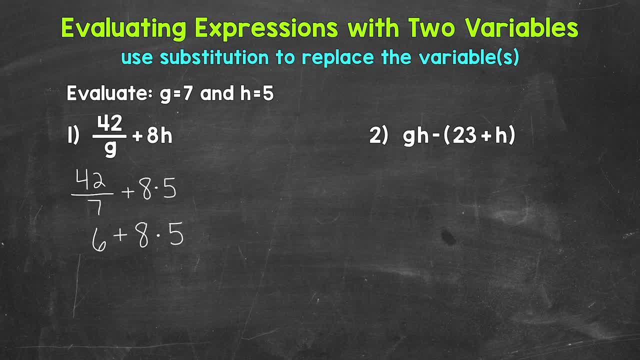 So the addition sign, the 8,, the multiplication sign and the 5.. Now we have addition and multiplication. Multiplication comes before addition, So let's multiply next 8 times 5, that equals 40.. Bring down the addition sign and the 6 that we did not use. 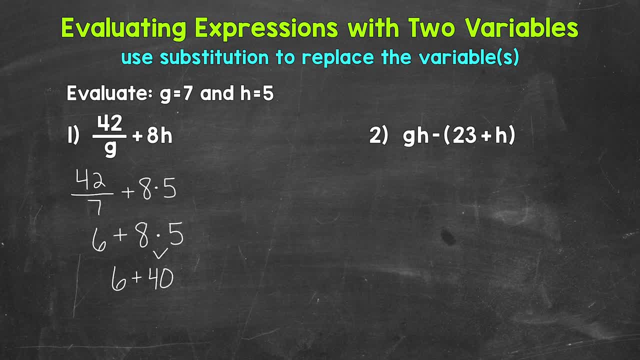 And we end with addition. So we have 6 plus 40. That equals 46. So the value of this expression is 46 when g equals 7 and h equals 5.. Let's move on to number 2, where we have gh, So g times h. 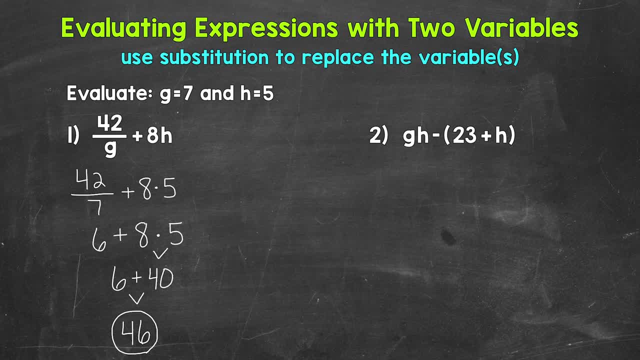 minus and then in parentheses, 23 plus h. Let's plug in and evaluate. So we start with g, Let's plug in 7 for g times h. Plug in 5 for h minus parentheses, 23 plus h. So plug in 5 and then end parentheses. So now we need to go through the order of 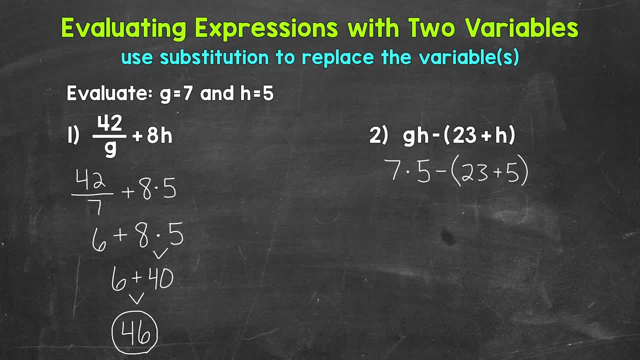 operations in order to evaluate this expression. Do we have any parentheses? Yes, So that is priority number 1.. So let's go through the order of operations in order to evaluate this expression. Let's start there. We have 23 plus 5. That equals 28.. Bring down everything we did not use. So 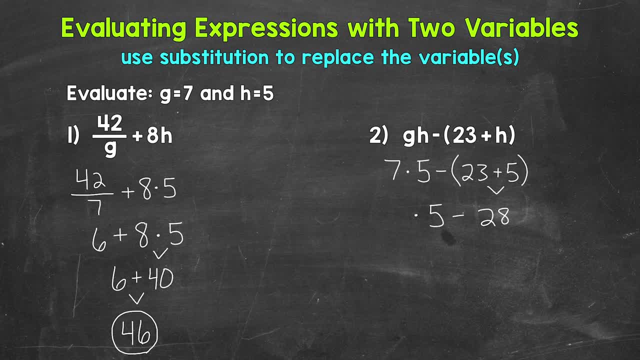 the subtraction sign, the 5,, the multiplication sign and the 7.. So now we have multiplication and subtraction. Multiplication comes before subtraction, So let's multiply next: 7 times 5, that equals 35.. Bring down everything we did not use, The subtraction sign and the 28.. So we end.